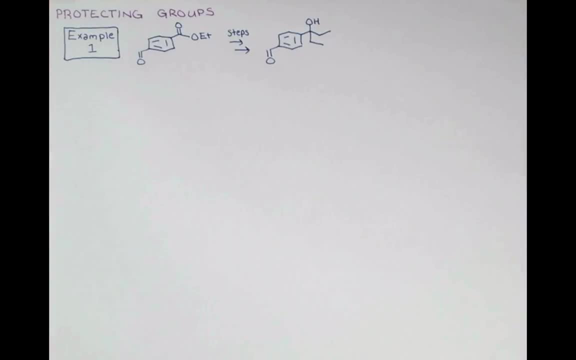 on the molecule and we want that to remain as an aldehyde throughout the course of the reaction. First, let's devise our general reaction sequence. that'll allow us to perform this reaction and get our tertiary alcohol. Now that we're focusing on just this piece, 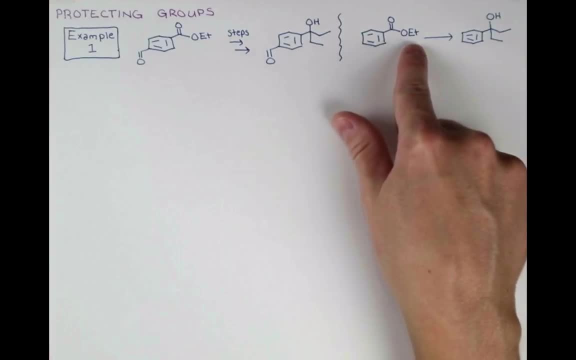 of the molecule. we're going to go ahead and do a little bit of a test. We're going to see that we need the O-E-T group to leave. We also need to add in two ethyl groups, And a great way to add in a carbon nucleophile, to add an alkyl group into a molecule, is by 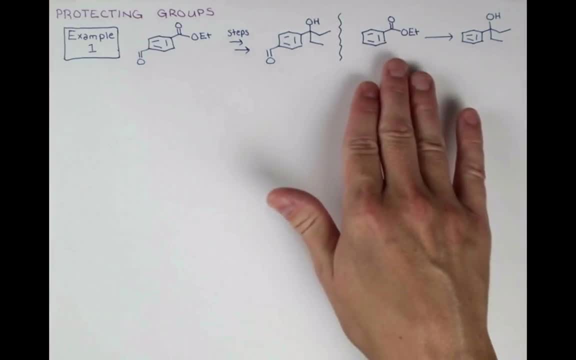 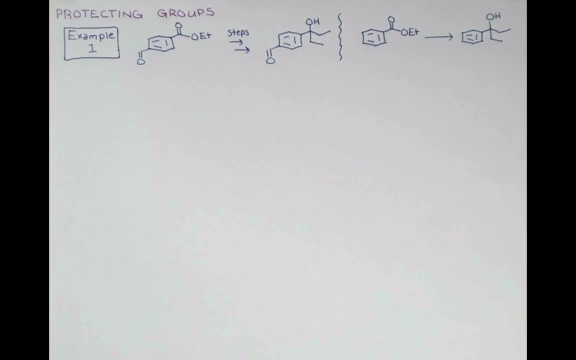 using a Grignard reagent. Esters actually will smoothly react with two equivalents of the Grignard reagent and then a protonation step will give us this alcohol. here I'll draw out the intermediate after the first equivalent of Grignard reagent and then a. 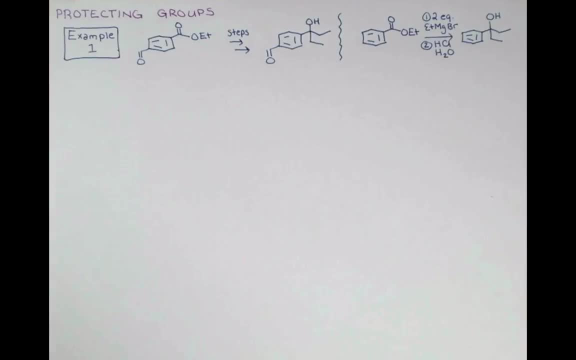 fraction of the Alkyl reaction in equation two here, including the горilline constant which we've already discovered in ocean Tran debt. Then If you stir up your nucleophile and see that the nickel group O-E is lost to all olefate and D-L, then 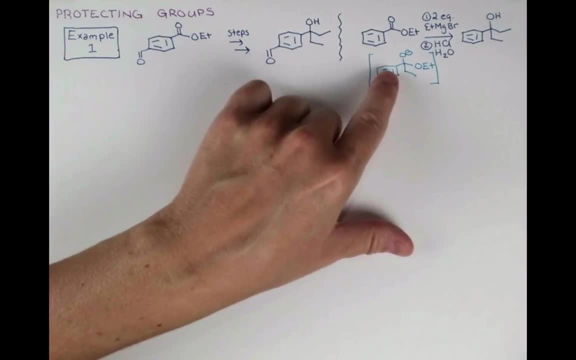 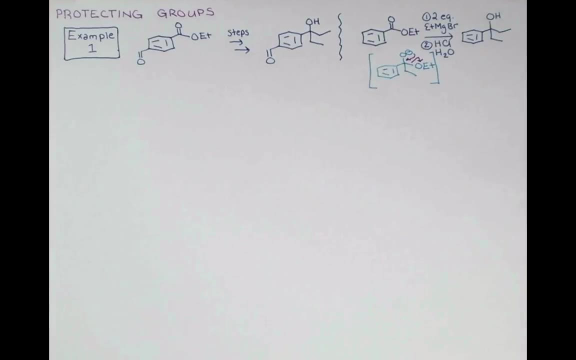 think you've run out of charms over here. You don't have enough 밀 Niye. How do you run that down at this point? What's theazaing brine of all you've got? Well, you're gonna run it up right away. So have you tried ridding with Яnol Titanol離? 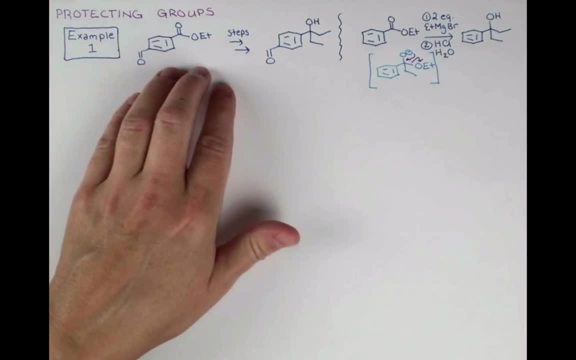 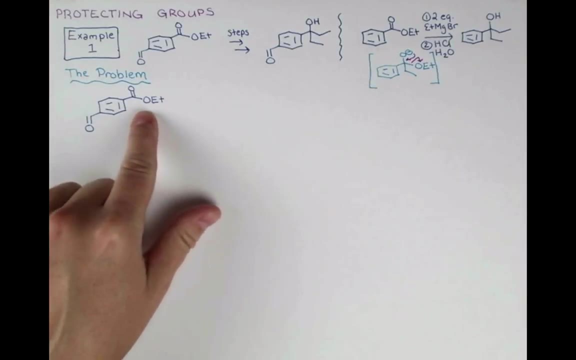 е, You're gonna lose. Okay, we've got twonumber O-E. I've already said I don't feel we've to this transformation here. Well, the problem is that the ethyl ester over here is not the most reactive part of the molecule. 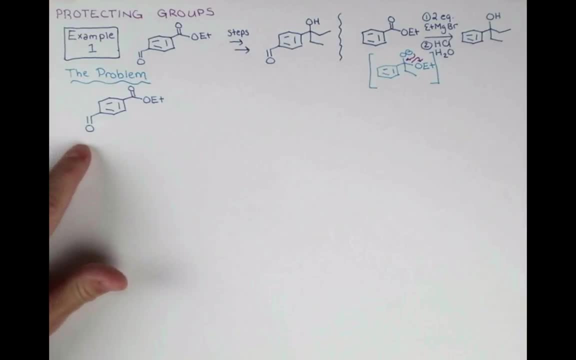 We have this aldehyde and this aldehyde is prone to attack. It's even more reactive than the ester. The ester has resonance from the lone pair on this oxygen. that's actually stabilizing this functional group. The aldehyde doesn't have a group over here, just a. 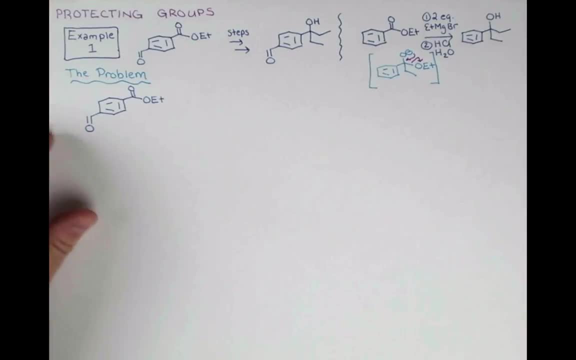 little small hydrogen atom, And so it's not very sterically hindered. it doesn't have the stabilizing resonance, so actually our aldehyde will want to react first, and it'll do so more readily than our ester. So here's our complication drawn out. We're doomed to get mixtures. 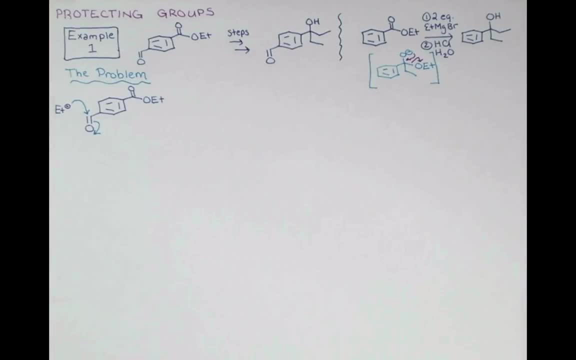 of the ethyl group adding in over here and some over here. Our solution is to use a protecting group to mask this aldehyde. There are three criteria for a protecting group: It must be easy to put on, Then it must be unreactive. 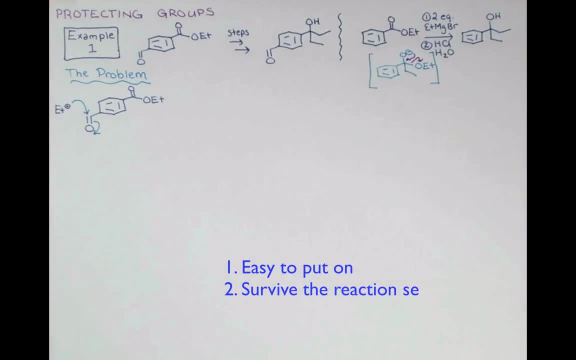 toward all the conditions that the molecule needs to go through. So every reaction that you put it on for it has to be compatible with it, And then in the end it should be easy to remove. For this problem we can use an acetyl. 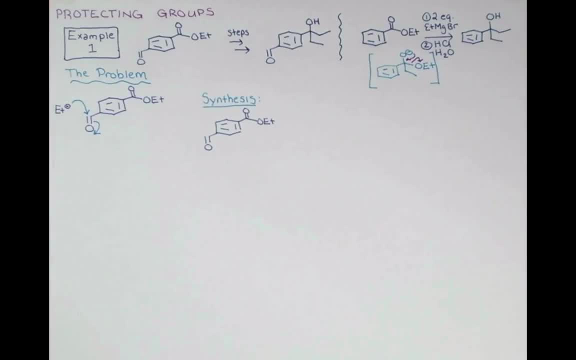 protecting group. Let's check out our synthesis Now. the fact that the aldehyde is much more reactive than the ester doesn't doom our synthesis. it's actually an advantage for introducing the protecting group If we treat this molecule with this diol ethylene. 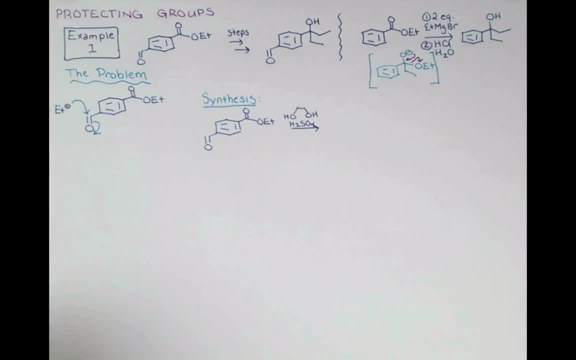 glycol. in the presence of acid, this group is more reactive, so it will react to form an acetal protecting group and the ester will stay in this form. The acetal is a base, stable protecting group that is removed in acid, so we put it on using acid, then we 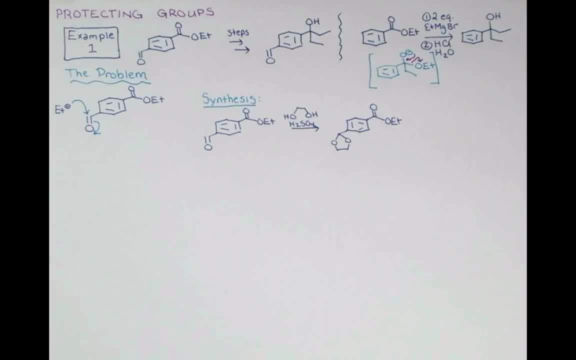 can remove it by acidic hydrolysis Since it's base stable. we can now apply these conditions above, and the acidic conditions of our workup might just be enough to remove this protecting group too. So in this first step the reaction happens where we add in our ethyl group twice. 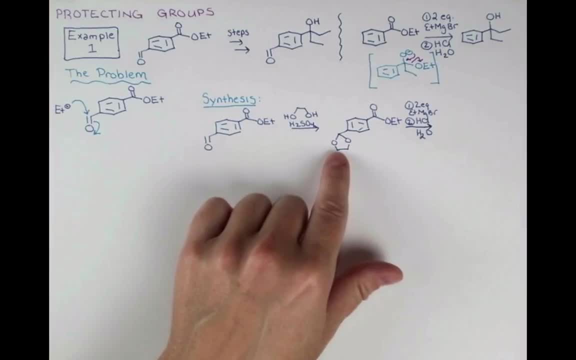 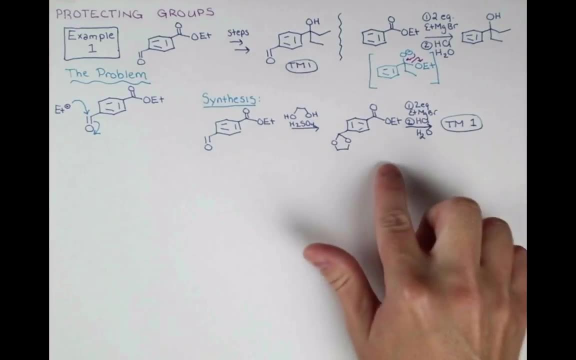 and then, when we're protonating this, we might be able to just heat it up and remove our protecting group at the same time. Let's call this target molecule one, and we form that by this sequence, using the acetal protecting group. Let's check out another. 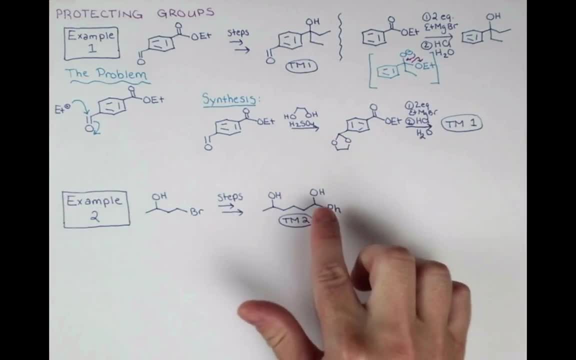 example. In this example we're also forming an alcohol and we're reacting this piece of the molecule. this maps on over here and we're adding a new alcohol and a phenyl group. It might benefit us to think about where we're breaking this molecule. do a little. 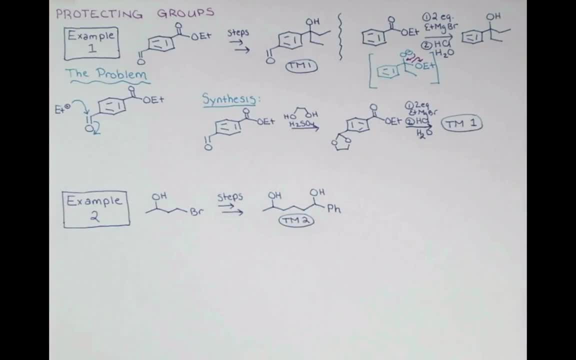 electrosynthesis to see the pieces that we might have to put together to actually form this. So over here we have one, two, three, four carbon atoms. So if we go one, two, three, four, we'll see that we need to cleave the molecule here. Well, when I see 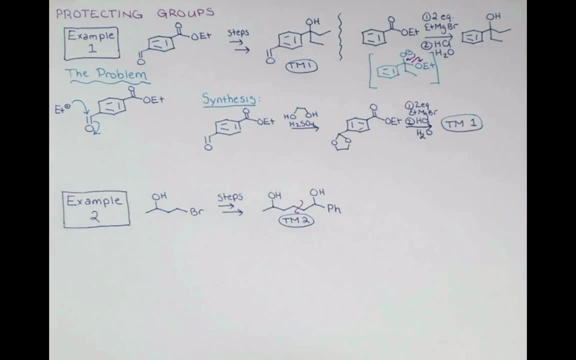 a bromide, I think Grignard reagent. Let's take a moment to look at synthons, the hypothetical electrophiles and nucleophiles that we would use to form this target molecule. Over on this side, we were talking about forming a Grignard from this bromide, So this would 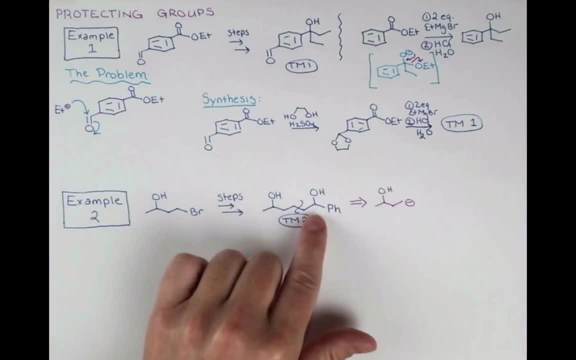 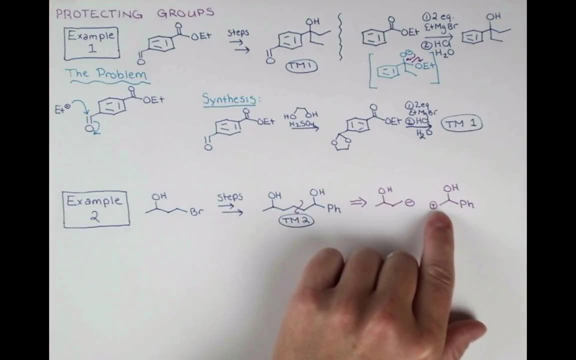 be our nucleophilic piece. Now let's consider what this side would look like. This fragment would have to be our electrophile, with some positive character on this carbon. But a thing that we can think about is, when we have an OH group next to a carbocation, what would 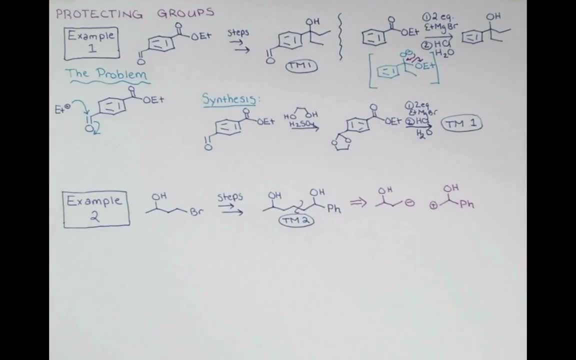 that look like if the oxygen donated in its electrons and formed an electron. Well, that's a bond. The reagent that we would use would be this epoxide, And Grignards very smoothly open at the least sterically hindered side of the epoxide. So we'd expect this to attach. 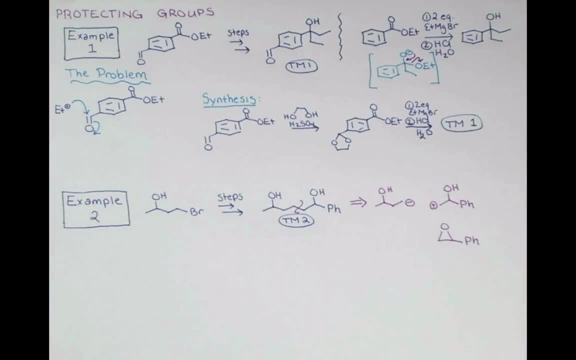 over here just like we want. So that's awesome. We have a synthetic route in mind now. So what's the problem here? Let's imagine we take this compound, treat it with magnesium metal and make a Grignard. So we might imagine this Grignard starts to form. but this is actually a self-destructing 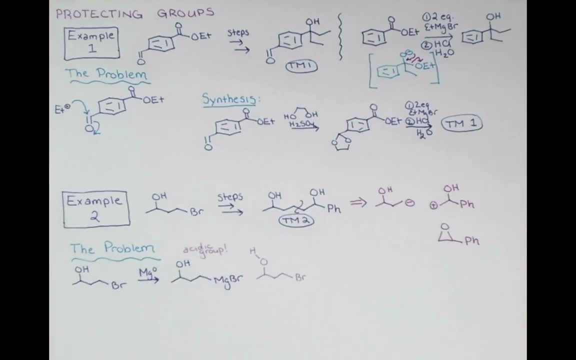 Grignard. There's an acidic group right here, So before this Grignard could ever attack and open an epoxide forming a carbon-carbon bond, it will instead react with an unreacted molecule of starting material, deprotonating this alcohol here and destroying the nitrogen. 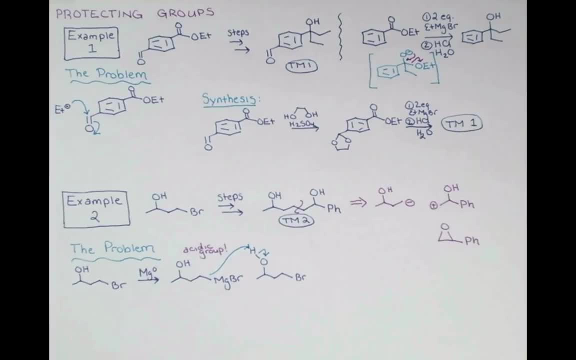 So we are going to take our Synthase to the Grignard before it can even do its job. So our Synthase must incorporate a protecting group for the alcohol. this time We can protect our alcohol with this silicon group. Chlorine is going to act as a leaving group here, and 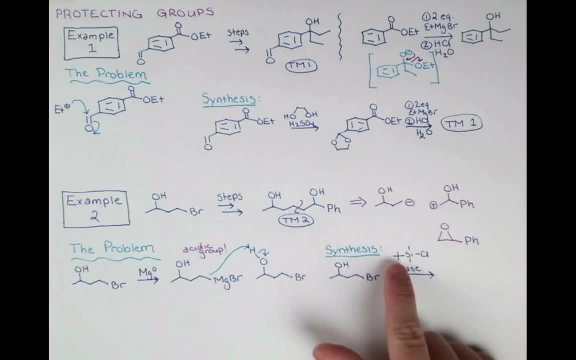 we'll put this group onto the molecule. This group is tert-butyl-dimethyl-silyl-chloride and is sometimes abbreviated TBDMS-chloride or more commonly, TBS-chloride. The chlorine in the Chlorine group is a very common choice of chlorine. Chlorine is sometimes used as a 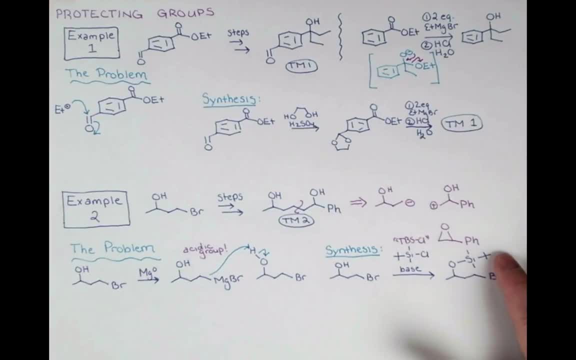 chloride, So we get this whole big group on here. The group is base stable. The base in this reaction is an amine base, so it just takes that proton off after. the TBS group is on the alcohol And a commonly used base in this reaction is 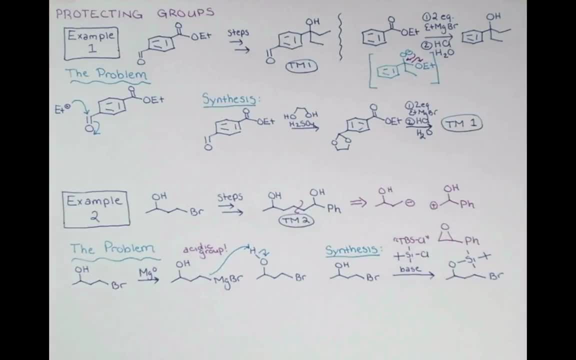 imidazole. Now we don't usually draw this whole group on here. Let me just show you how we would abbreviate this structure. Now that this oxygen contains a base stable protecting group, we can go ahead and form a grignard here and attack this. 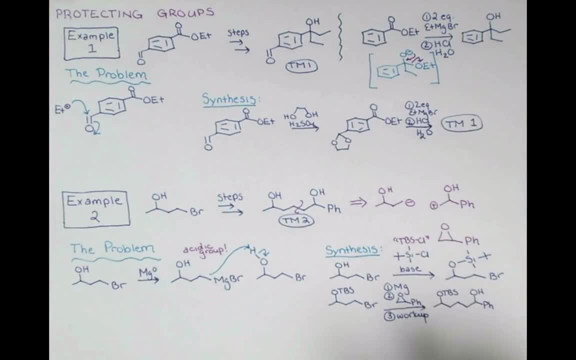 epoxide. Now, if this workup is acidic, that might knock off our TBS group, right then, and so we might kick off the TBS and free up our alcohol. However, we're gonna say it did not here, and I want to show you the standard conditions for. 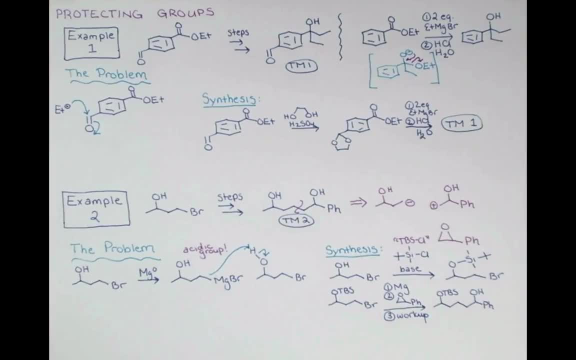 removing a TBS group, which is a fluoride compound called TBAF. This is a fluoride salt, tetra butyl ammonium fluoride, and it looks like this. So the F minus of TBAF comes in attacks at silicon forming a complex and then 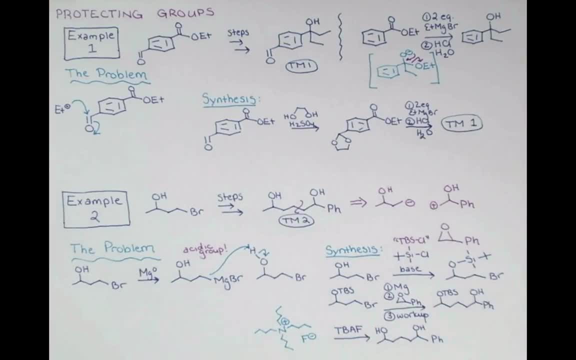 this group is removed from the molecule. Let's just summarize how this met the three criteria of a protecting group. This was pretty easy to put on. We just needed this compound here in the presence of a base, probably imidazole, and we were able to put the silicon group onto our oxygen. It was stable when. 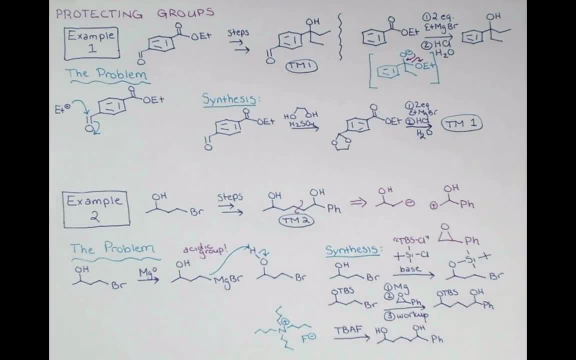 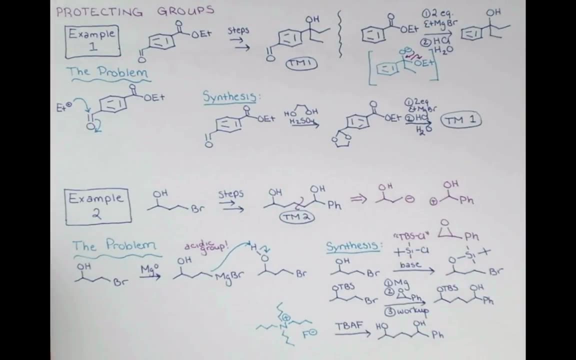 we formed a grignard over here and used that to open this epoxide, and then it was easily removed with TBAF. So far in this lesson we looked at protecting groups for aldehydes and ketones. The acetal is a. 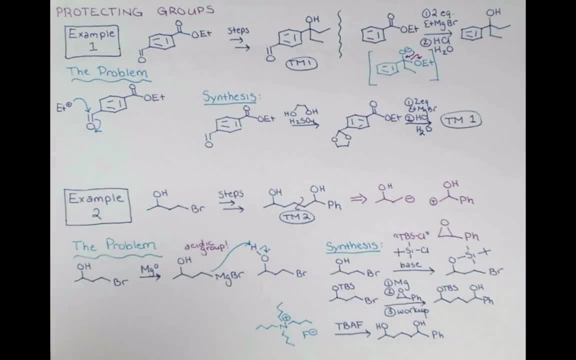 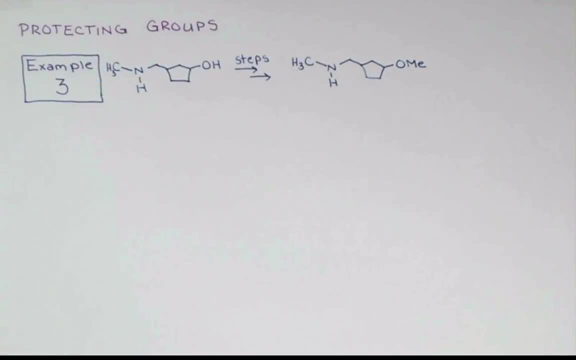 good one. We also looked at how to protect an alcohol from deprotonation by nucleophiles and looked at the TBS group. Another group that we commonly need to protect is amines. So let's take this third example. We're looking at the. 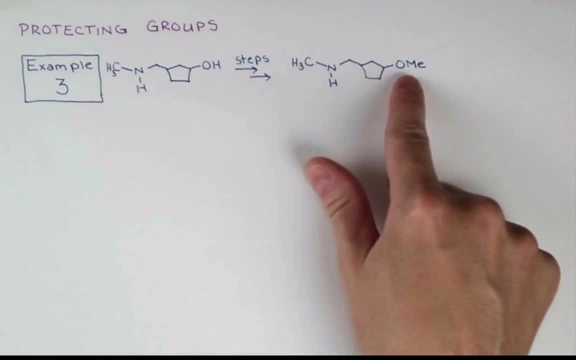 alkylation of this OH group. so we're adding a methyl or a CH3 here and we're leaving this nitrogen unreacted. First, let's just ignore the amine over here and look at what we would need to use to turn this alcohol into this methyl group. 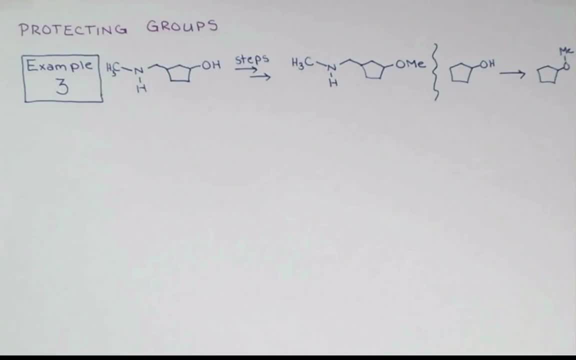 We can use a reaction called the Williamson ether synthesis, where we first deprotonate this hydrogen atom here and then we alkylate with something like a iodomethane. A great base to use for this reaction is sodium hydride. This will 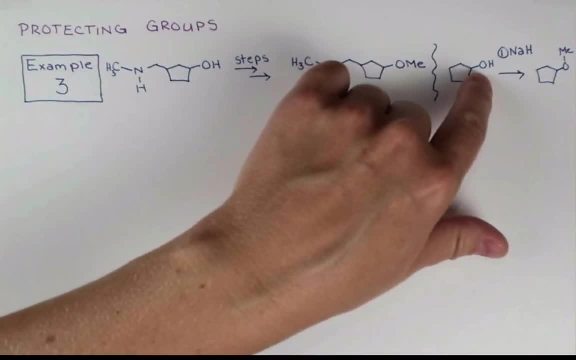 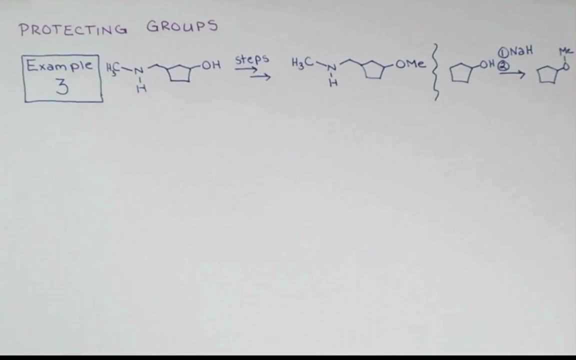 deprotonate our alcohol completely, forming an alkoxide, and as a byproduct produces hydrogen gas which bubbles out of your reaction. Then, in a second stage of this reaction, in the same flask, we can treat this with methyl iodide and. 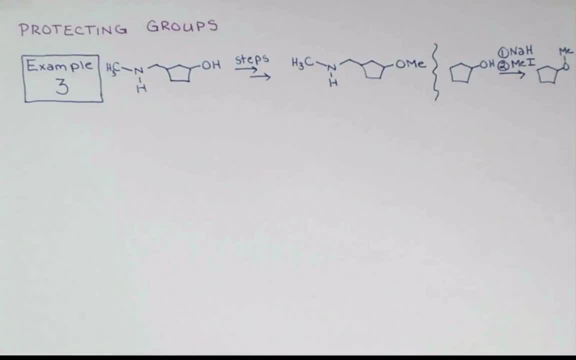 that'll alkylate our oxygen over here, giving the methyl ether. So what's the problem with having the nitrogen on there? Well, amines are great nucleotides, So in the presence of iodomethane, the nitrogen would be more likely to. 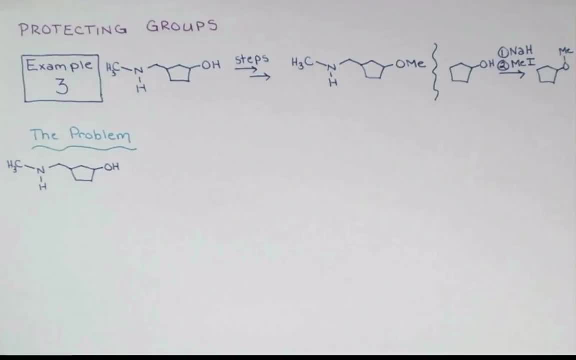 attack becoming alkylated than the OH group. But over here we talked about deprotonating this. so maybe we could just deprotonate with sodium hydride and then we'd have an alkoxide which is nice and nucleophilic and maybe we could. 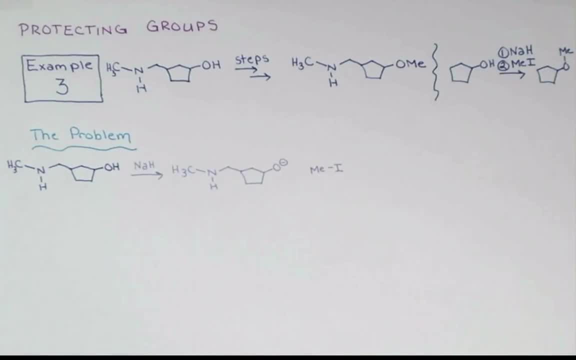 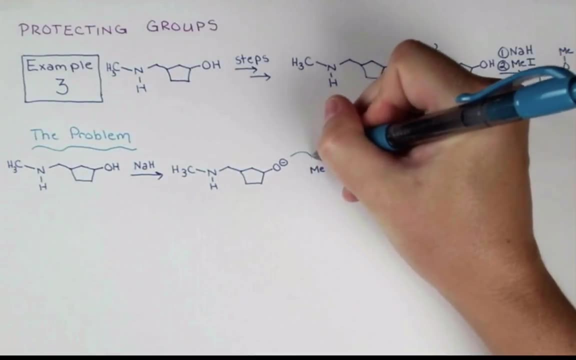 solve our problem that way. Let's see what would happen if we tried that. Well, certainly our alkoxide wants to react with the methyl iodide, so this would attack displacing iodine. Once we form this, we actually still have. 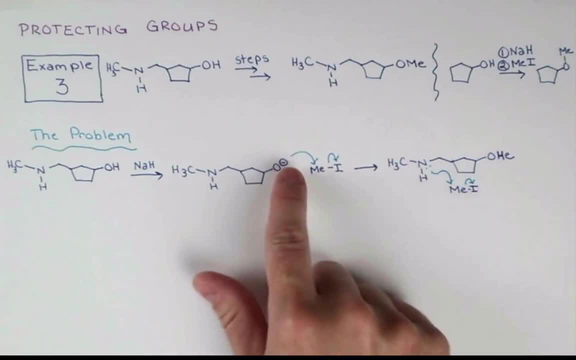 a nucleophilic nitrogen in the molecule, and now we don't have our alkoxide to be the better nucleophile, This is going to go ahead and alkylate, kicking off the iodine, and so we're still going to get mixtures of alkylation at the oxygen and 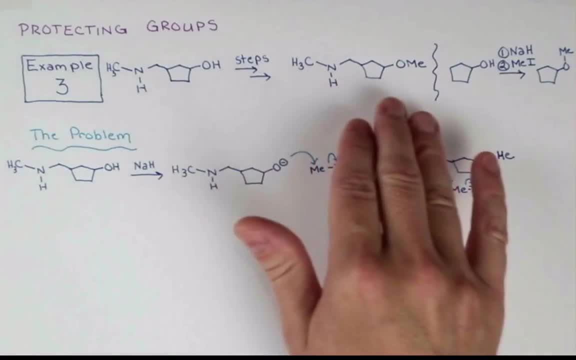 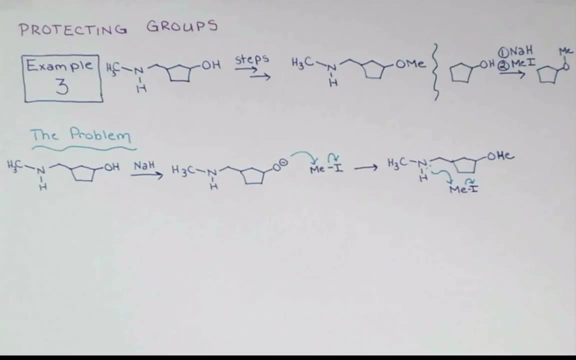 at the nitrogen, and so we won't be able to cleanly perform this synthesis where the nitrogen is unreacted. So what should we do? You guessed it: We need to protect our amine. Amines are more nucleophilic than alcohols, not the deprotonated. 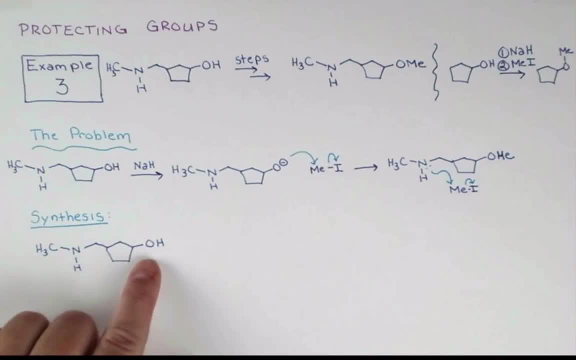 alkoxide, but more so than the alcohol itself. so we can capitalize on the nucleophilicity of nitrogen to introduce our protecting group. This protecting group is diterbutyl dicarbamate. It's an anhydride, but also a carbamate, because of all of these oxygen-rich molecules. 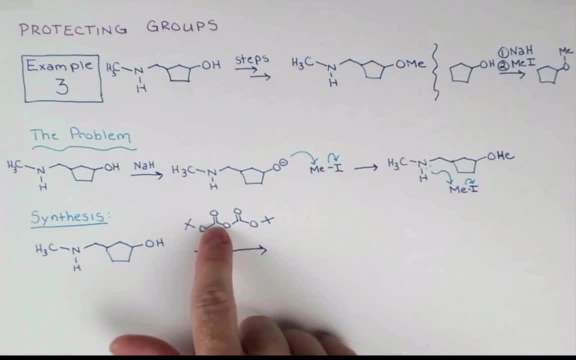 oxygens and the nitrogen is going to attack at this carbonyl, kicking off all of this group. Fortunately, just like that big TBS group, we have an abbreviation for this one as well: We call this BAC anhydride and we write the abbreviation like this. So the BAC is representing this part of the. 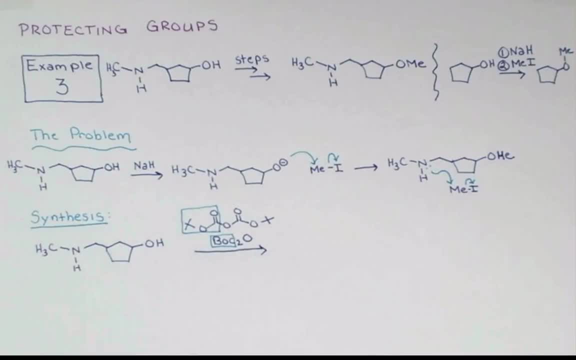 molecule. So we have two of them and an oxygen in the middle. Nitrogen attacks here, forms a tetrahedral intermediate. We kick off the rest of the molecule and we get this structure. Here it is with our abbreviation, and let me draw it out below Now. the nitrogen is a carbamate functional. 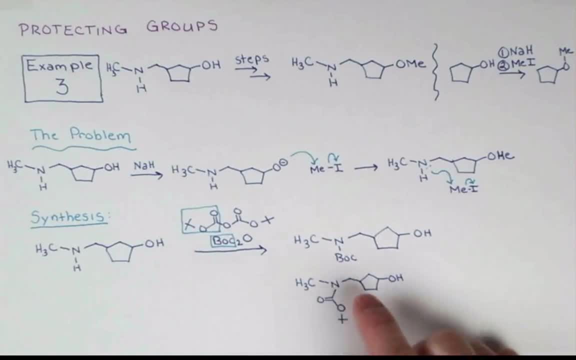 group. That's what it is when it has the nitrogen carbonyl oxygen. Like an amide, this nitrogen has lots of resonance with this carbonyl. Thus the lone pairs that would have attacked iodomethane in that alkylation step are now tied up in resonance. 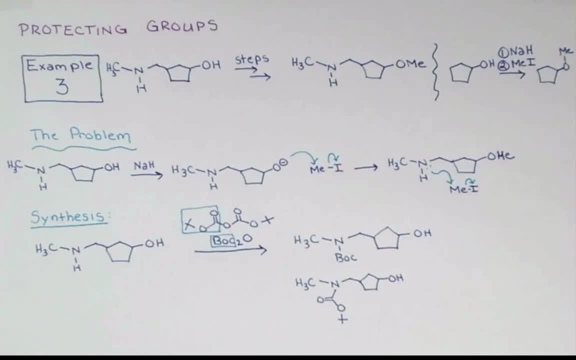 Making the nitrogen less reactive. It's protected because it is not as nucleophilic anymore. Now let's deprotonate our alcohol and alkylate Now. our BAC group was stable during these basic alkylation conditions. Notice, it has a carbonyl, so some nucleophiles could mess with the BAC group. 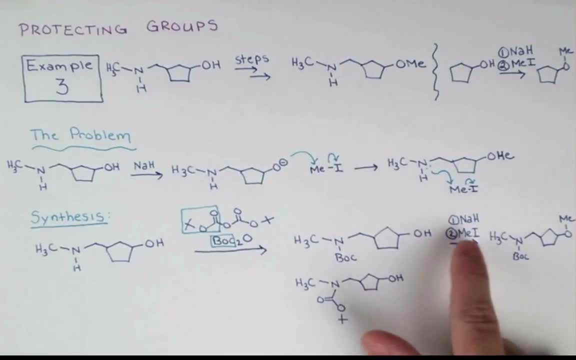 maybe grignards and things like that, But under these alkylation conditions it's just fine. The BAC group is most commonly removed under acidic conditions And the preferred acid for this reaction is trifluoroacetic acid or TFA. And if we call 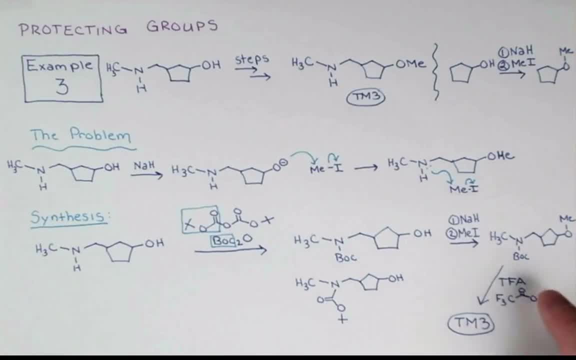 this compound target molecule 3, that's what we get from this deprotection. Under acidic conditions this group is removed as a tert-butyl cation and so sometimes there's problems with alkylating other groups with that cation. that's in solution, but there are other additives to work around this. 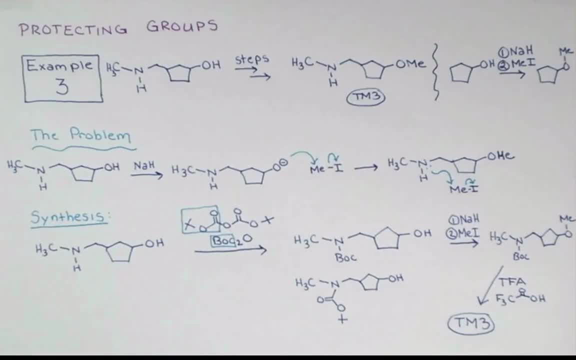 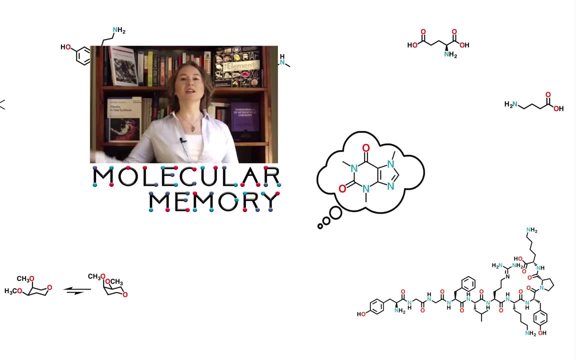 Organichemistryorg has some nice tables on protecting groups, so I'll put a link to that in the video description. Thanks for watching and have a great day KP here. If you learned something, give me a thumbs up on the way out. and for more chemistry, subscribe to my channel.